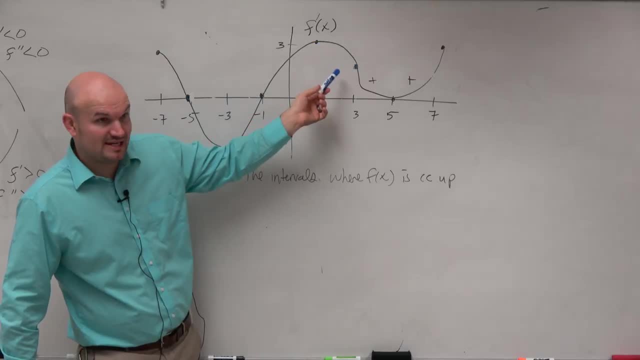 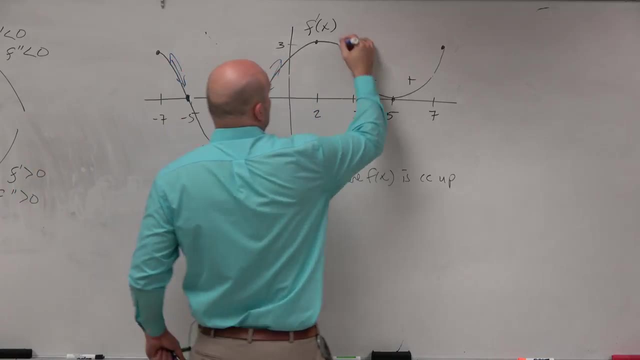 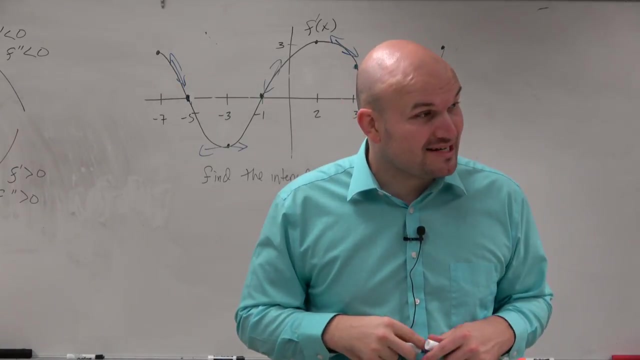 So the second derivative is basically the slope of this. So we have all these slopes like you have a slope line here, slope line there, slope line there. If we're looking for concavity when it's concave up, we're looking for when the second derivative is positive. 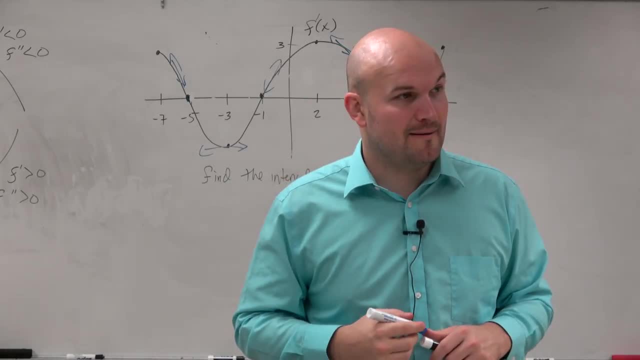 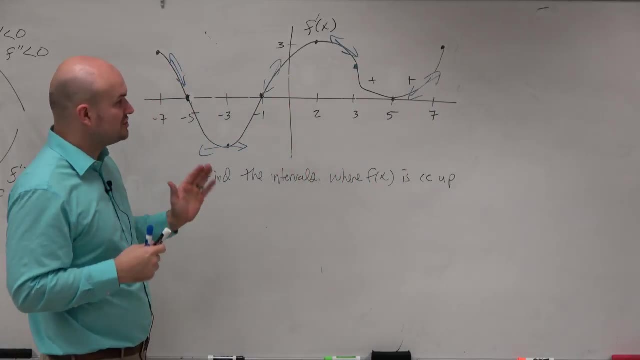 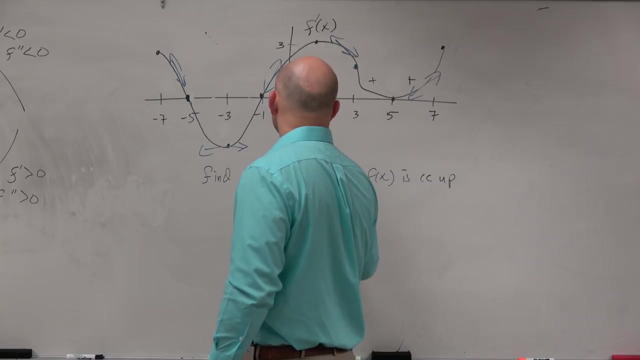 That means the slope of the first derivative is positive. We want to find when the slope of the first derivative is positive. So we see that there's only two values or two intervals where the slope of the first derivative is positive, We could say that the derivative is going to be from negative 3 to 2.. 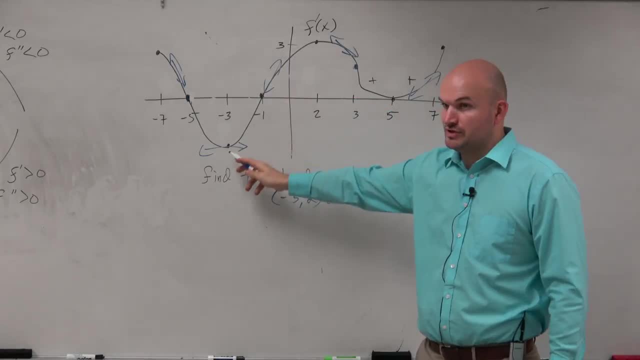 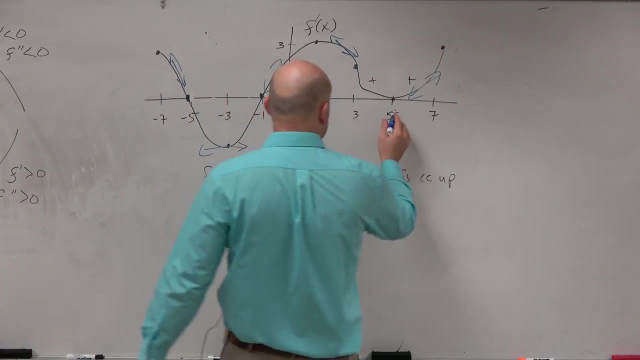 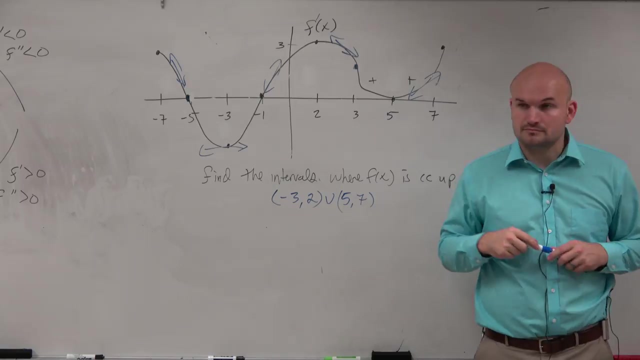 We agree, guys, that the slope of this function, of this first derivative, is positive. That means the second derivative is positive on that interval, And we could say from 5 to 7 is also positive, because that's where the slope is. 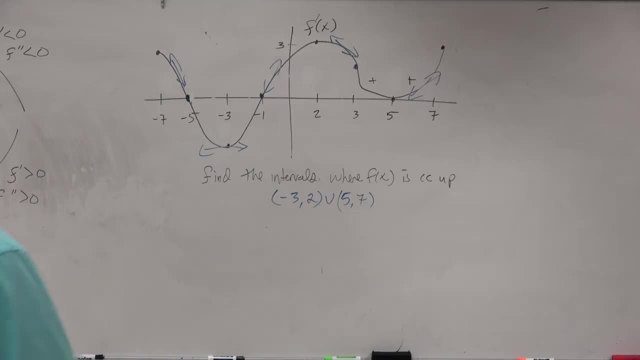 positive on that first derivative OK. 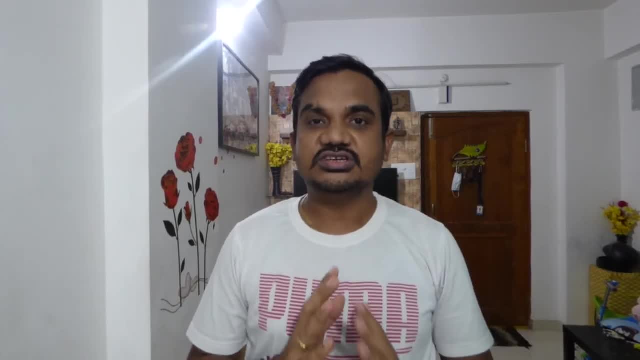 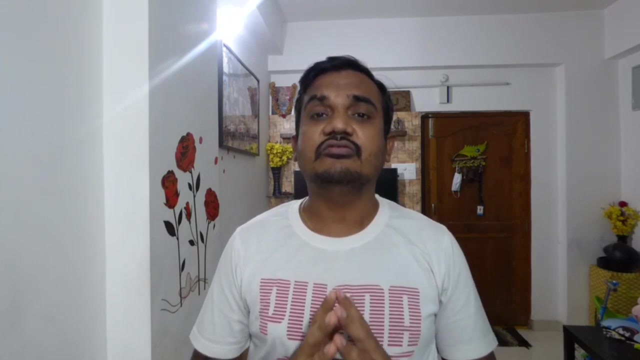 Hello friends, welcome back to another video of Automation Testing Insider. So today I'm going to talk about an important software development model that is Agile model. You can call it as Agile development process model, Agile process or Agile methodology, And this is a very important software development model which is widely used and frequently used by different software development companies. And this is you should be aware of what is the Agile process. Every QA must know about this process.